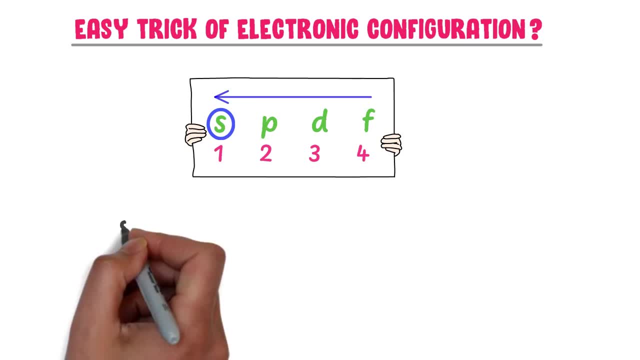 So I take S and write it 2 times: S and S. Let me repeat it: I take S and write it 2 times S and S. Secondly, I go from P to S. I take P, S and write them 2 times: P S and P S. 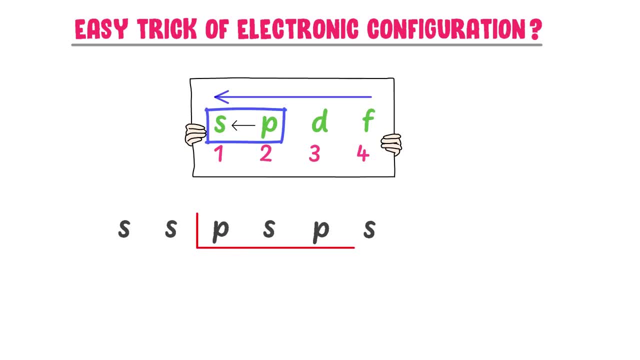 Let me repeat it: I take P S and write them 2 times: P S and P S. Thirdly, I go from D to P and then to S. I take D P S and write them 2 times: D P S and D P S. 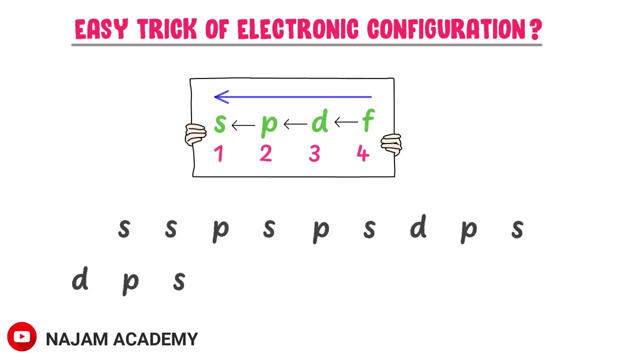 Fourthly, I go from S to S. I take F to D P S. I take them and write them 2 times: F D P S and F D P S. Now listen carefully. S is the first orbital, so start numbering S orbitals from 1.. 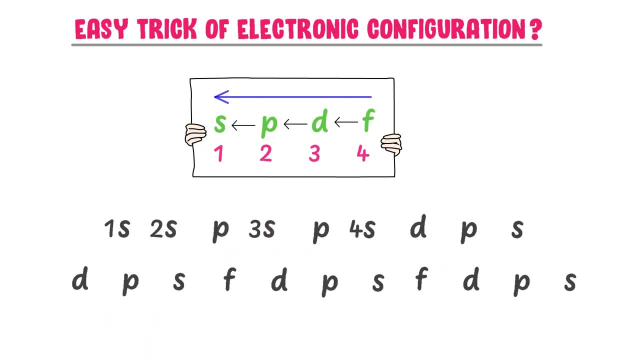 Hence 1 S, 2 S, 3 S, 4 S, 5 S, 6 S, 7 S and 8 S. P is the second orbital, so start numbering P orbitals from 2.. I take D P S and write them 2 times: F D P S. I take D P S and write them 2 times F D P S. Hence 1 S, 2 S, 3 S, 4 S, 5 S, 6 S and 8 S. I take D P S and write them 2 times: F D P S. 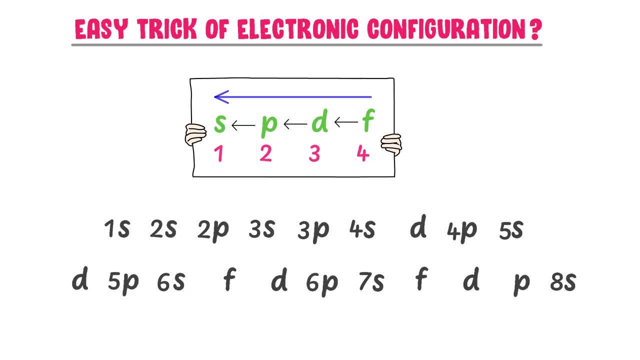 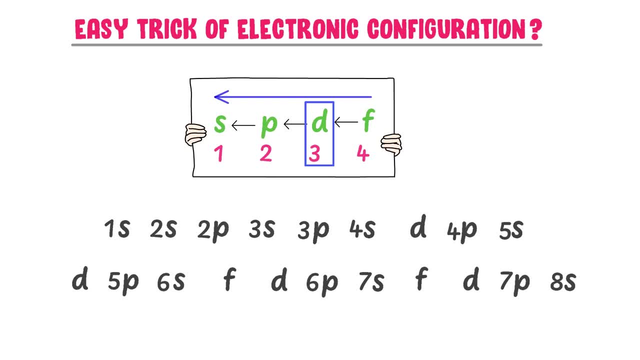 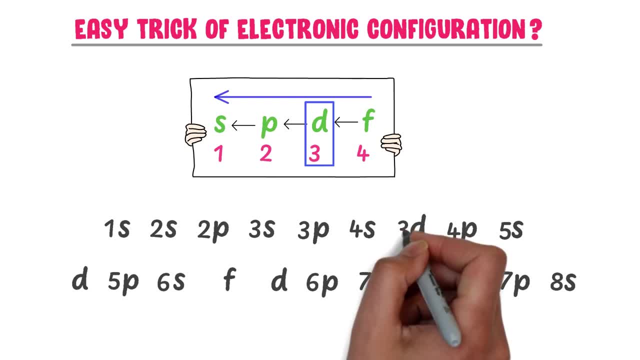 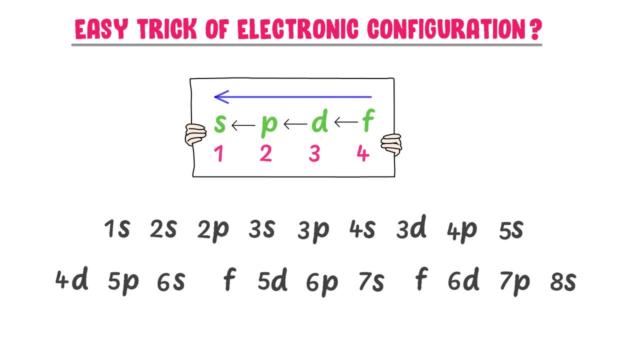 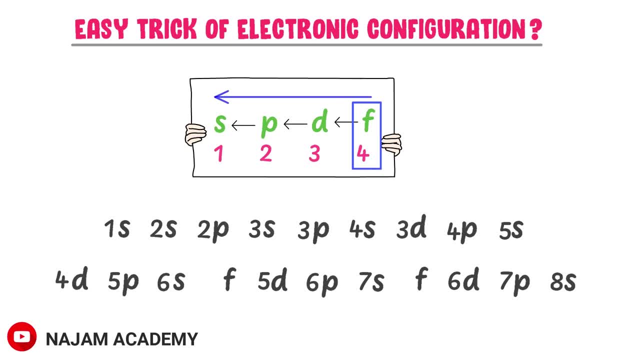 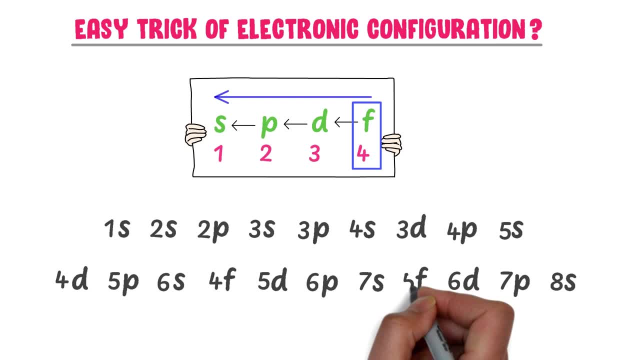 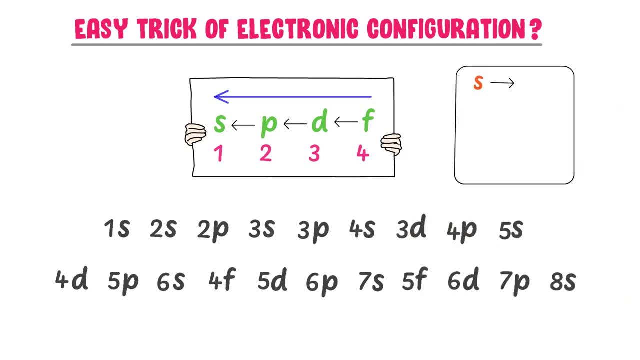 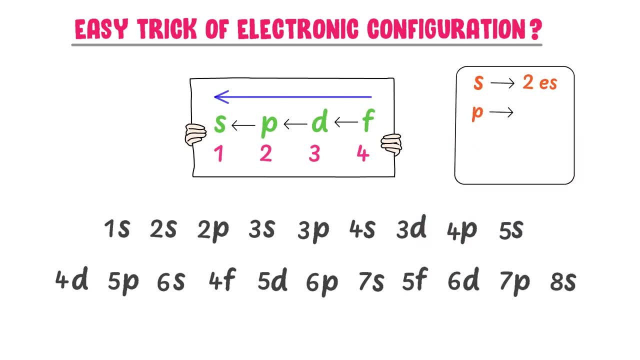 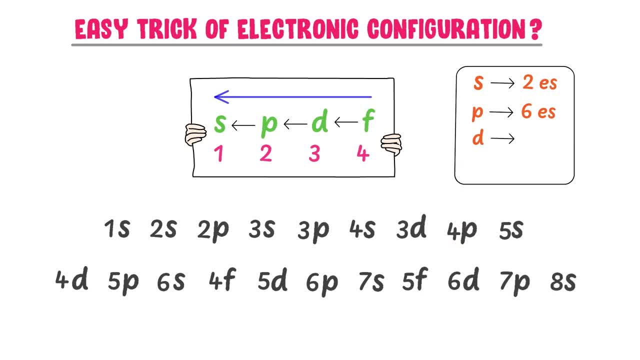 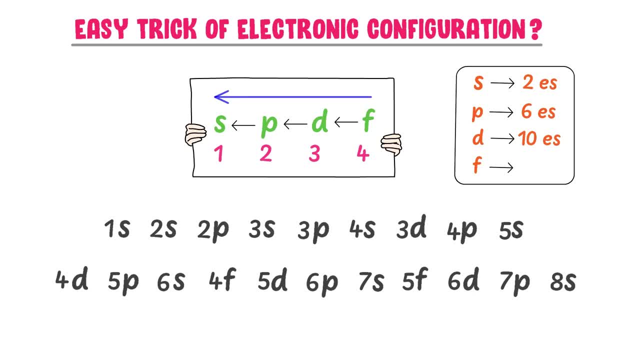 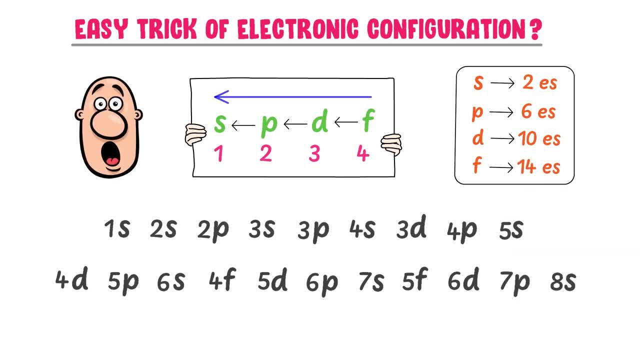 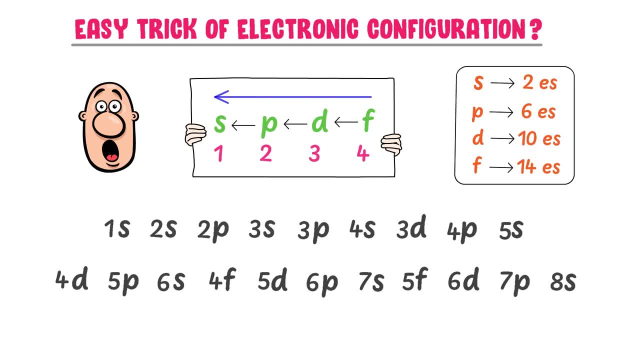 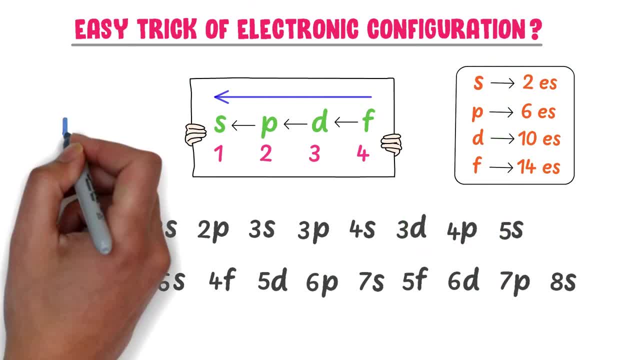 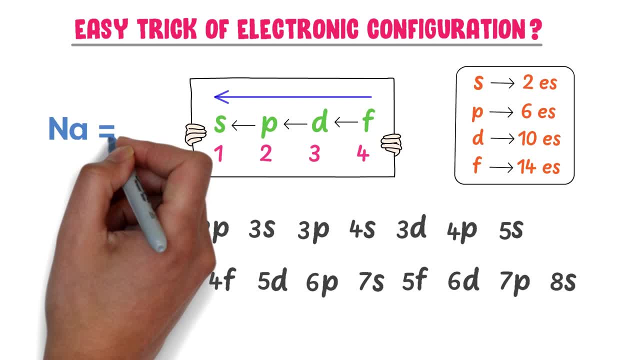 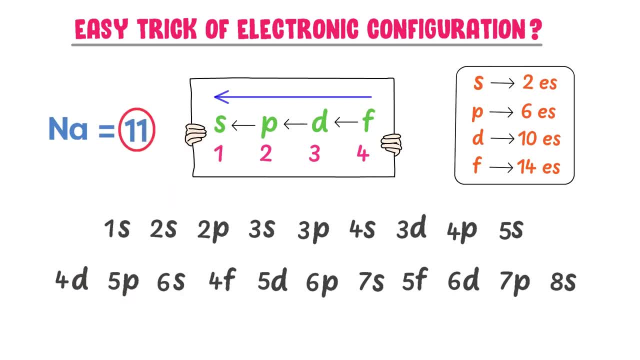 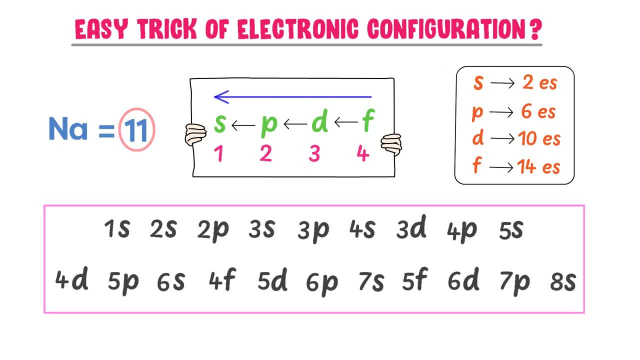 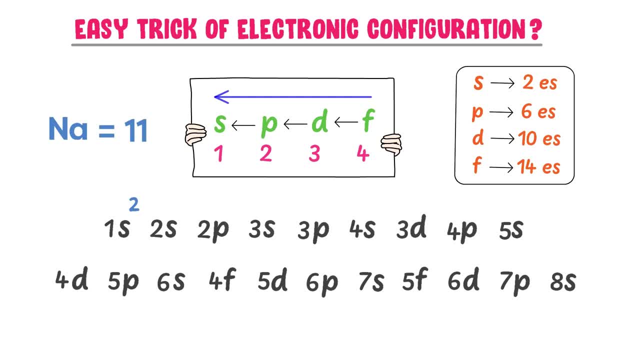 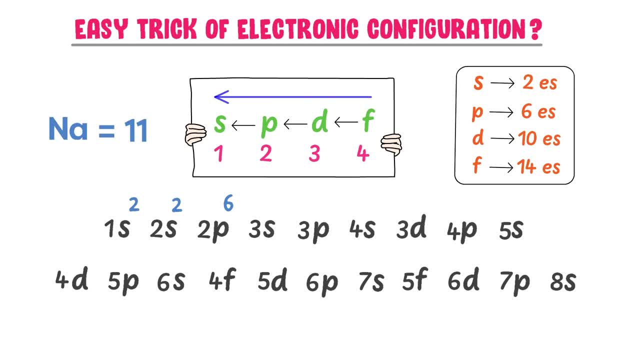 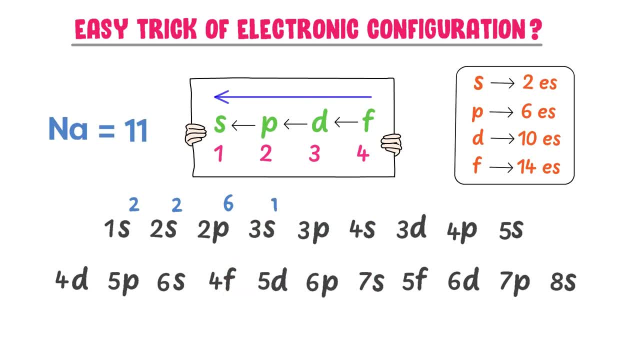 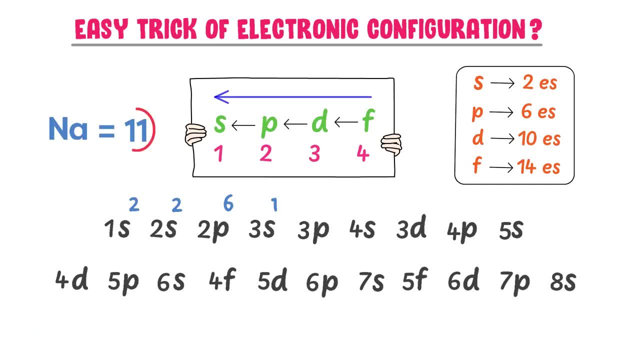 So I have accurately distributed the 11 electrons of sodium and this is the SPDF electronic configuration of sodium. The last electron of sodium is an S orbital, so sodium is also called S-block element 1s 2 electrons, 2s 2 electrons, 2p 6 electrons, 3s 2 electrons, 3p 6 electrons, 4s 2 electrons, 3d 10 electrons and 4p 5 electrons.